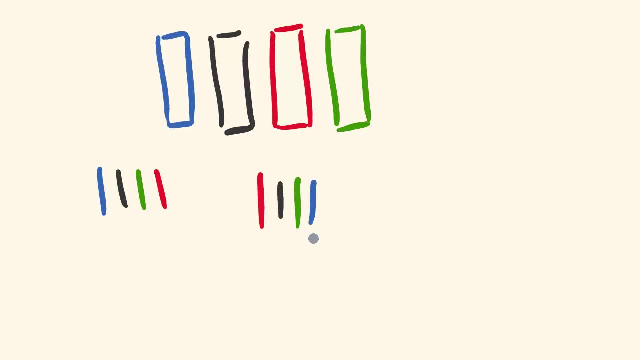 And this is what these combinations and permutations start to look at. And, more specifically, today, this is what this counting principle will be looking at. Okay, and we're going to be using this in some later parts of what we're going to be doing. 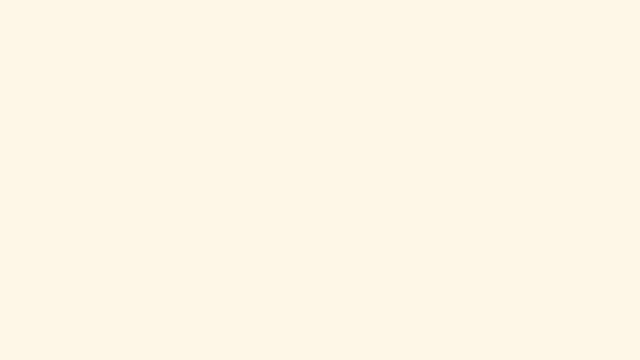 So we're going to explain this by going through an example, And we're going to start by imagining I'm choosing my outfit for the day. So, anyway, I look in the cupboard and the first thing I look down at is my shoes. 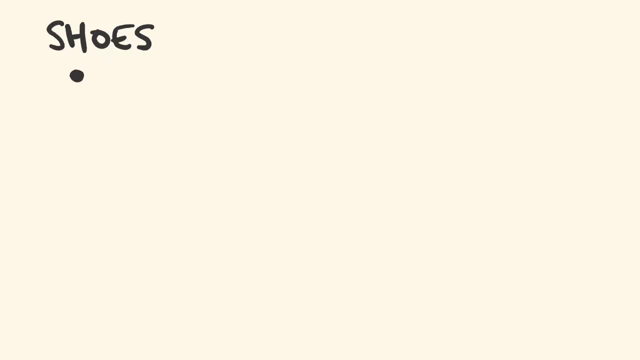 And I'm trying to decide what shoes I have to wear. I have black shoes and I have blue shoes, Okay, Okay, and then the next thing I'm going to decide is what colour pants I'm going to wear for that day. 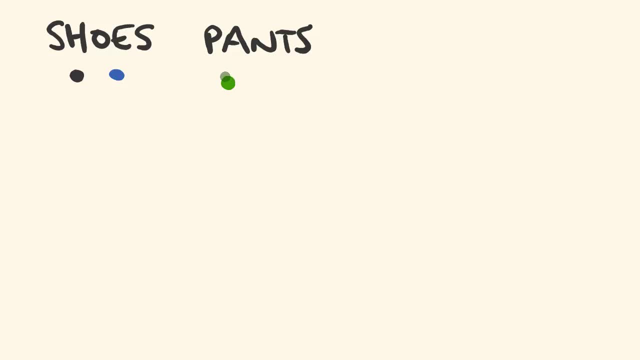 And because I'm a funky sort of guy, I have green pants and I also have orange pants, And then the next thing I'm going to decide is what shirt I'm going to wear. Okay, so I think to myself: I have a red shirt, I have a blue shirt and I also have a black shirt. 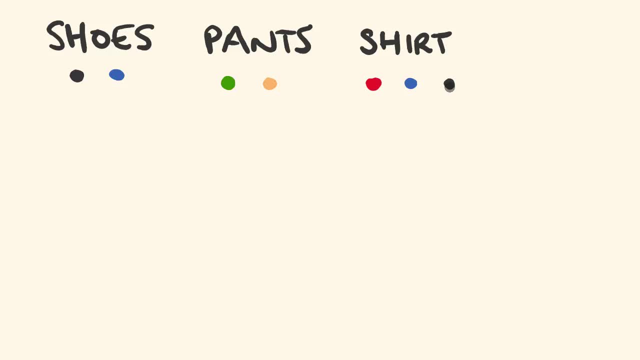 And so, how many different combinations of outfits, How many different combinations of clothes can I wear out of these? shoes, pants and shirt combinations could I make out of that? So this is where we use this counting principle to work out. 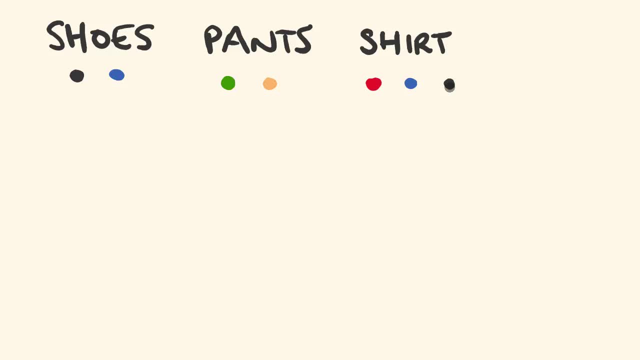 But first off, what we're going to do is we're going to draw up a tree diagram. Now, a tree diagram pretty much lists up all the different combinations that are possible. So we look at all the different decisions that we make. 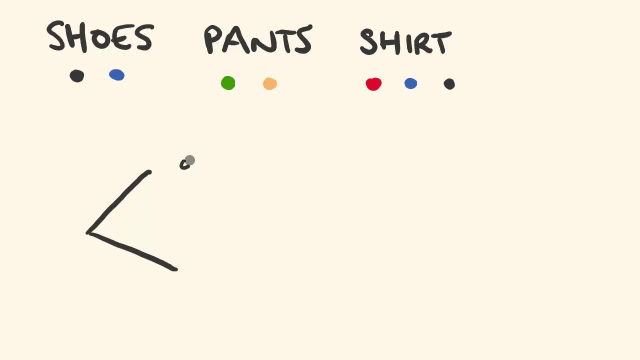 So the first decision we make is what shoes I'm going to wear. Now we could either choose that I'd be wearing black or I'd be wearing blue, So we have a different branch that goes off to each of those. 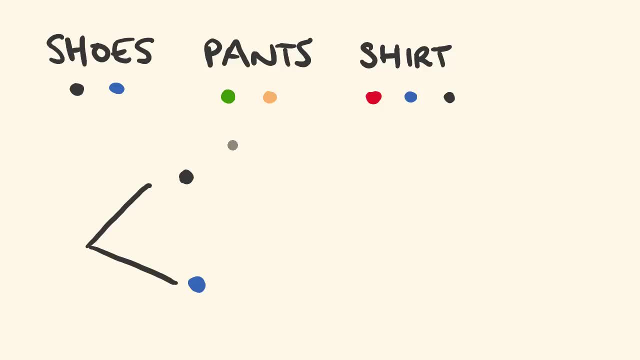 The next thing we decide is what colour pants. So for each of these I might then decide: I'm going to wear either green, so this one I could wear black and then black shoes and then green pants, or blue shoes and then green pants, or I could use wear orange pants with either of these decisions. 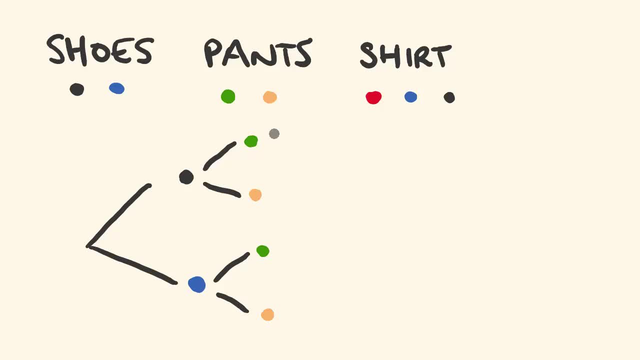 The third thing I then do is look at shirts. I could wear blue, Three different colour shirts- for all of these, yeah, So I could wear a red shirt, okay, or I could wear- you guessed it- blue, or I could wear black. 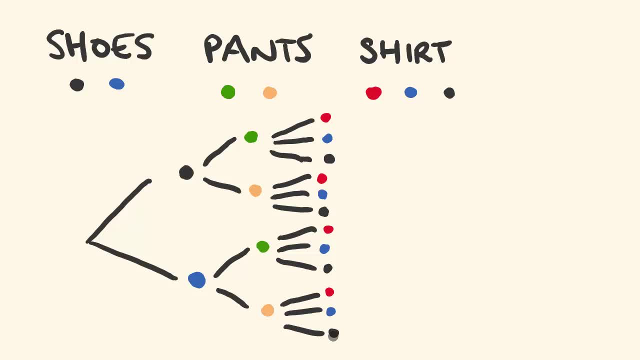 And so what this tree diagram does is it lists off all the combinations, and what you'll see is, if you count the ends of the branches here, you see how many different combinations we have. We have one, two, three, four, five, six, seven, eight, nine, ten, eleven, twelve combinations. 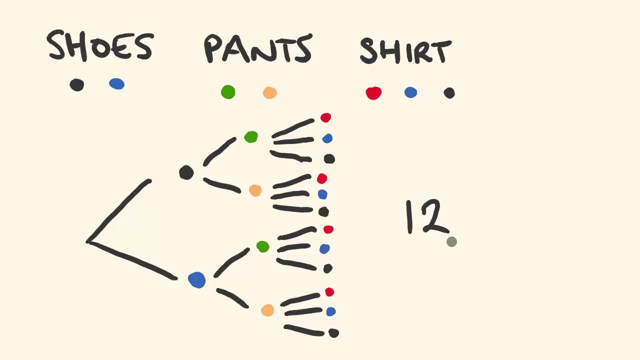 Twelve different combinations of outfits I could wear. And you're thinking to yourself: well, that's pretty handy-dandy and you'll look pretty funky if you wear various ones. but you might then think: is there a faster way of doing that without drawing out this tree diagram? 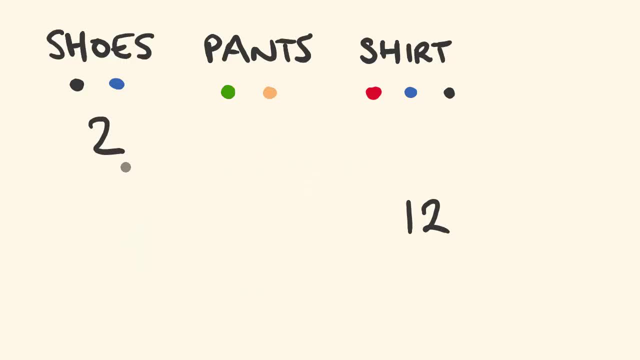 And there is- and I'm going to show you how to do that- because I have two pairs of shoes, two pairs of pants and three shirts and the very simple way of doing that is, if I just multiply these through Two times two is four. times three equals twelve. 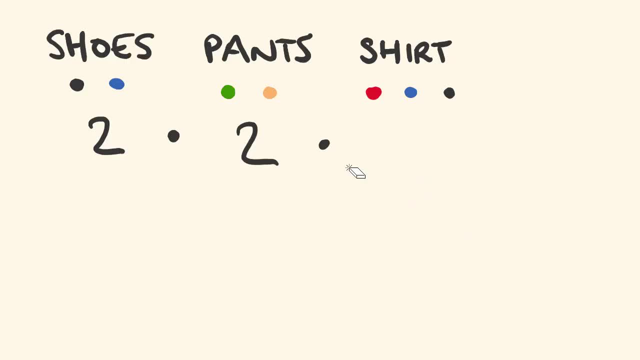 So say, for instance, I varied this up and all of a sudden now I have six pairs of shoes, I have seven pairs of pants and I have twelve pairs of shirts to choose from. How would I go about, rather than drawing one of those tree diagrams, which would take ages and, to be honest about it, would be rather squishy and not very fun to draw? 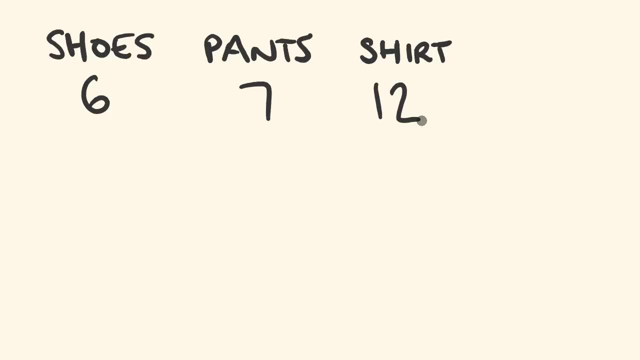 how would I go about doing this? Well, I just multiply this through. So how many different outfits could I have? Six times seven times twelve? Okay, so that multiplied together, mate, I have five. I'm taking this down and I need to do that. 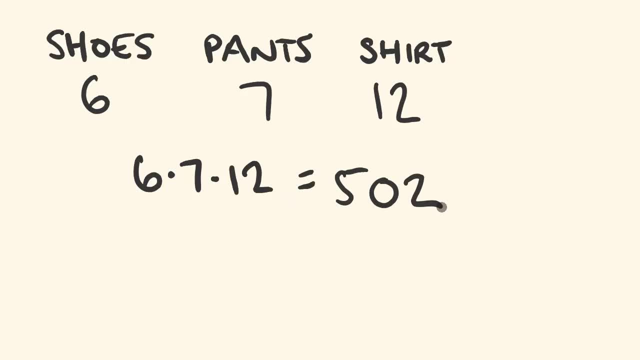 I need to do that. I need to make it bigger. I need to make a bigger one. I need to make it smaller. I need to make it bigger, I need to make it bigger. five hundred and two different combinations of clothing i could wear- okay, so that's a really. 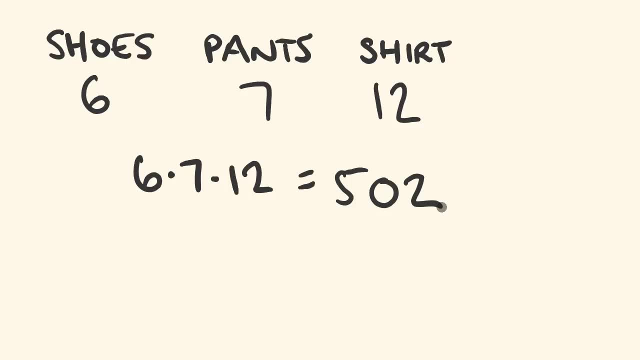 really easy way of doing this, um, and i could write out a rule for that, but i think you really probably just get that. you just get your number of different combinations and then you multiply. so what about you try some? so what about we have a menu? okay, you go in a restaurant, we have a menu. 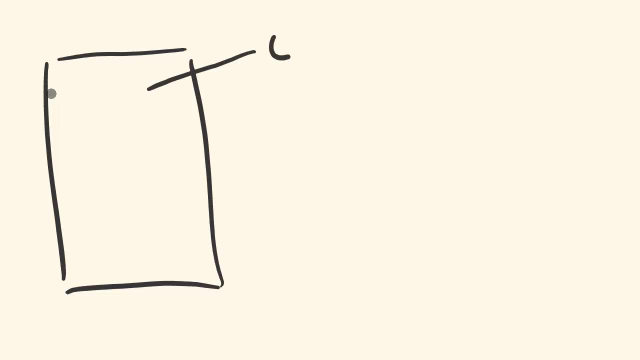 and on this menu, we have entrees, and there are four of these, and then, after the entrees, you have main course dishes, and then, on the desserts, we have three different types of desserts, and i could ask you then, how many different three course dinner combinations could you make off this? 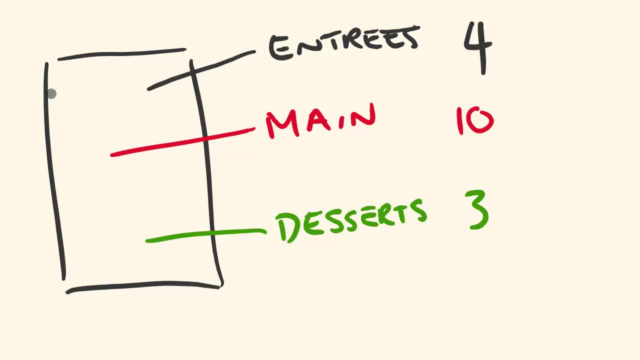 so i'll get you to work it out. i reckon you need probably, i reckon you should have already worked it out, because i know you're all great at multiplying and i think what you do is you go four times ten is forty times three. okay, that's going to be 120 different combinations. it's okay, a bit of a harder. 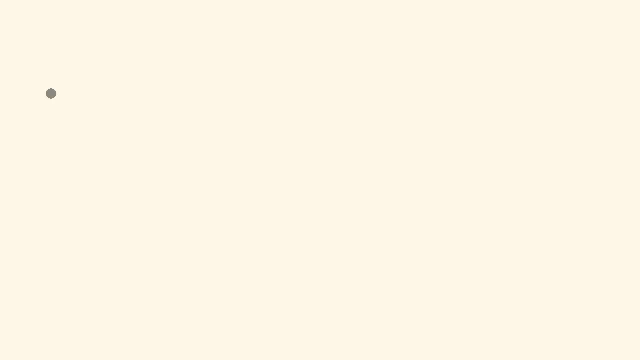 example now. so say, we have a lotto um where we have six numbers, so six numbers, and i'll draw them here: one, two, three, four, five, six numbers, and they get chosen from one balls numbered from one to 45. okay, and now i want to know is how many different combinations do we have here? 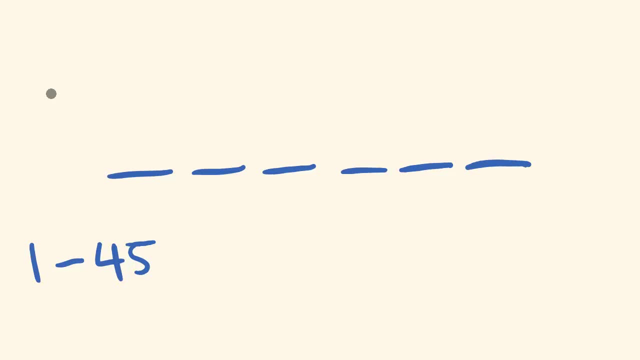 so this is a bit of a harder one, and the way that we do this is as follows. so i've got the slots here and this is a really good thing to draw. at the start there's six different balls we're choosing. i've drawn six different slots, so there's going to be six different things. we're multiplying. 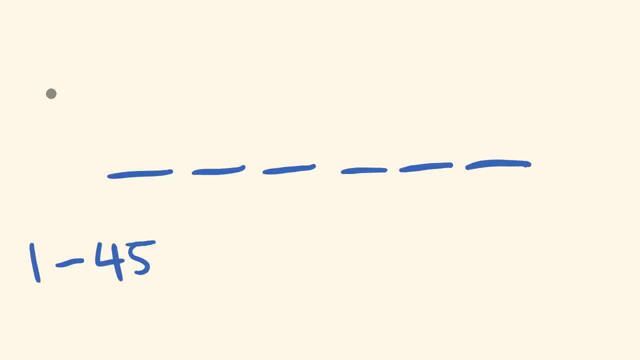 so the first slot here, the first ball we choose out. okay, we have 45 balls- 1 to 45, you might think of the first ball we choose out. we have 45 possibilities, anywhere from 1 to 45 that we choose for the second ball. 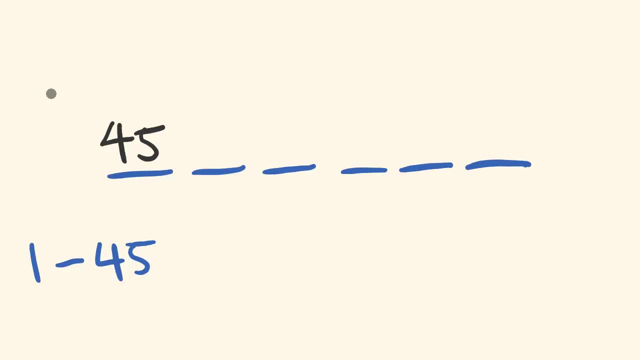 we choose out. how many possibilities do we have? well, one of these balls has been chosen out now, so we only have 44 balls left. so there'll be 44 different possibilities. okay, what about the next one? we'll have 43 possibilities, 42 possibilities. the next one had 41 possibility, because the ball 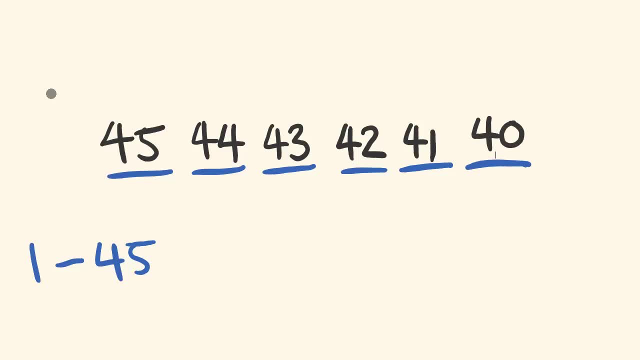 is gone and then, because that ball's gone, on the next one we have 40 possibilities. so how many different combinations do we have? and so you might look at this and think, okay, okay, how we work that out, we're going to multiply. that's a lot of numbers to multiply. we have the number of 5. 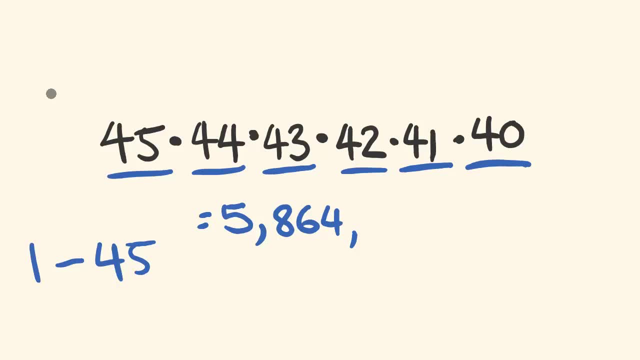 billion eight hundred and sixty four million four hundred and forty three thousand two hundred combinations. so one other one, and this one is a bit more where i come from. i come from victoria in australia. we have, well up until very recently we used to have license plates that were like this: we would have three letters say a. 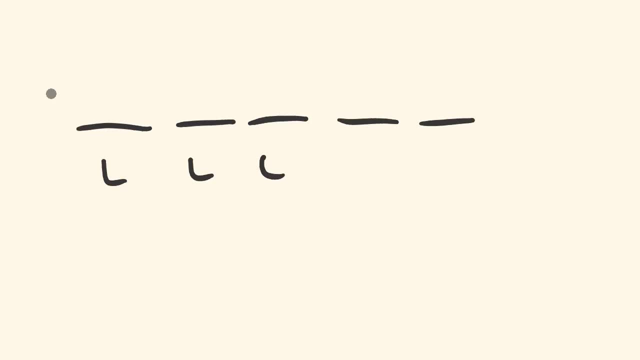 letter, letter, letter, and it was followed by three numbers, and i've been to different places around the world and i've seen that everyone has different types of license plates, but this is the ones we have and you could work this one out for your own license plates where you're from. so i want to know. 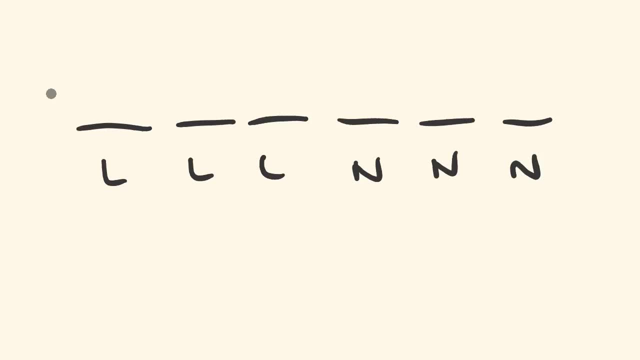 what combinations we have that we could have here. i mean, obviously it's going to be affected a bit. um, they don't like to have rude words and that sort of deal on license plates, but we're not going to take that into consideration. you know we're not going to have poo or anything like that. um, so how? 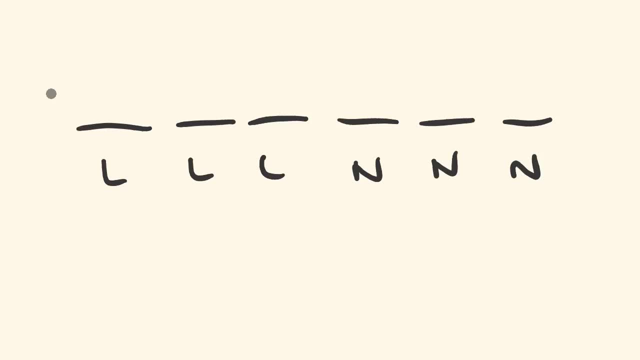 many different combinations license plates could we have. so you might think to yourself: okay, the first one, they could choose any letter. there's 26 letters in the alphabet, so there's 26 possibilities for that first letter, and then the next one- they could choose once again, any letter, because there's 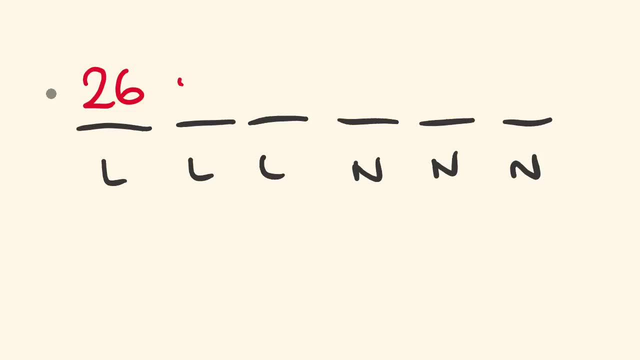 26 letters. you could have a and then you can have another a, so we're not worried about repeats here- and then the next one. you could also choose 26 letters out of 26 letters. now numbers: we have zero, one, two, three, four, five, six, seven, eight, nine. that's 10 different possibilities, 10 different and 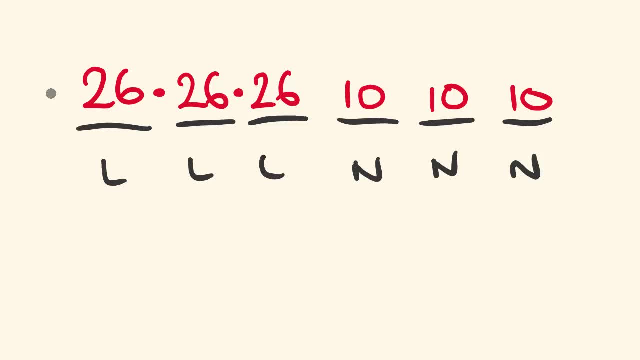 10 different for the next ones. so how do we work out? how do we count up all these combinations really quickly? well, we multiply them through. so 26 times 26 times 26 times 10 times 10 times 10, and the answer to this is there is 17 576 000 combinations. so you could work that out. 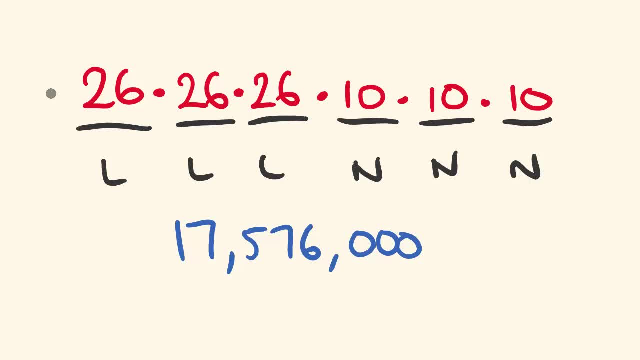 on a license plate where you're from, okay, and however, they work them out because they do vary. but i'm just going to finish with one last thing on this, which is this idea: so say, what about? are we worried about a license plate where we couldn't repeat any letters, or 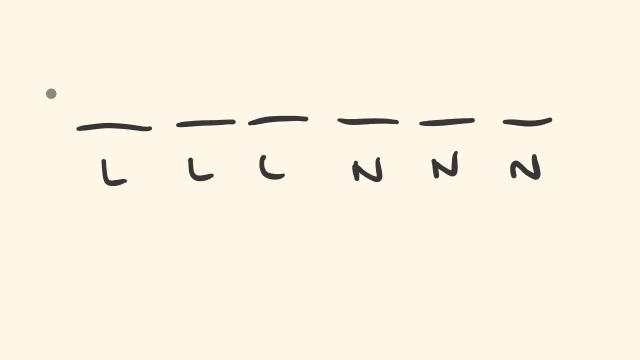 numbers. okay, every letter and number had to be unique. how would you work that out differently? that's not a huge thing to do, because of the first number of letters that came out, you would have 26. now say it was any number one of those letters that you took out, it would only leave 25 letters.